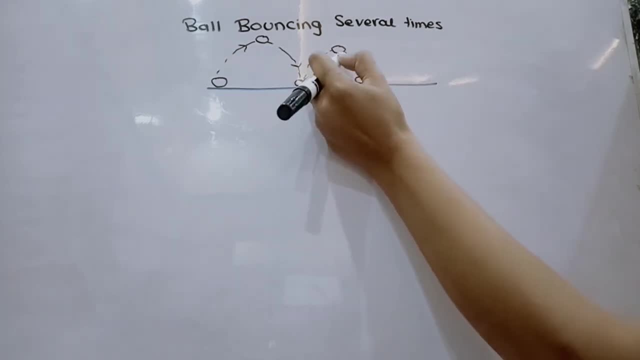 this, And the next bounce is again lower than the previous one, So that's the next bounce. Now for this. there are several things that we must note. One of the thing is that the height of every next bounce is less than the previous, and 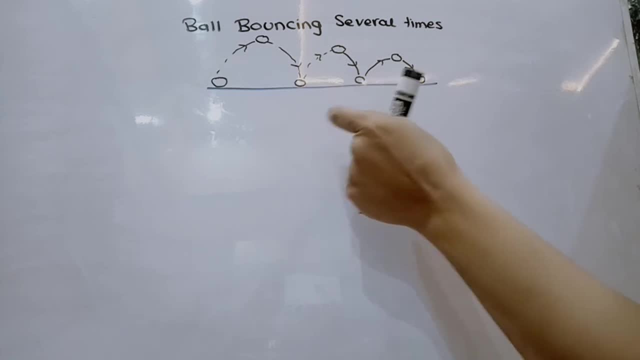 the time span after each bounce, it decreases. The reason behind this is that whenever the ball is in contact with the surface, there is always energy loss as a result of heat etc. And when there is an energy loss, the kinetic energy as a result decreases, because conservation 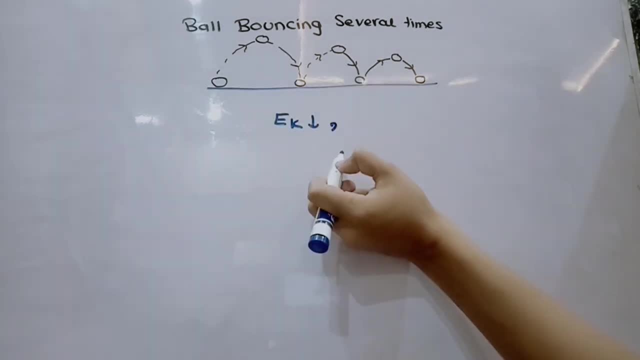 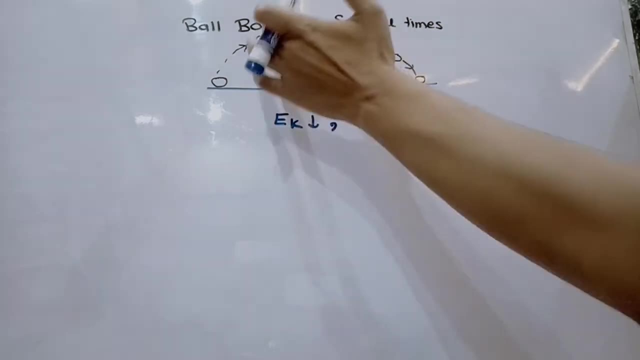 of energy is maintained. when the kinetic energy decreases, the velocity also decreases. So as a result, as a result of the kinetic energy, the potential energy decreases. so as a whole, we can say that the height decreases, the velocity decreases and we can say that this whole thing. 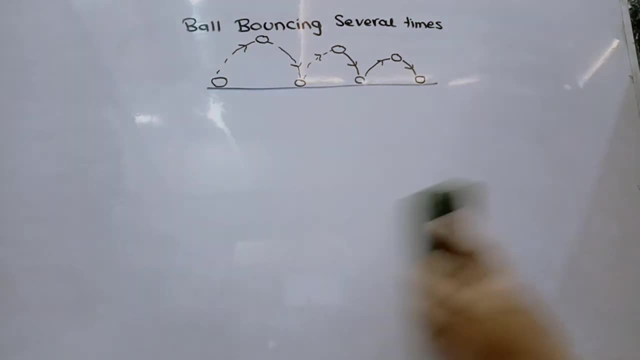 So that's it. Now. let's first sketch the velocity time graph for this and discuss that during what the velocity time graph will look, in which shape. So this is how our velocity time graph would look like for a ball bouncing several times, and each time the height decreases. 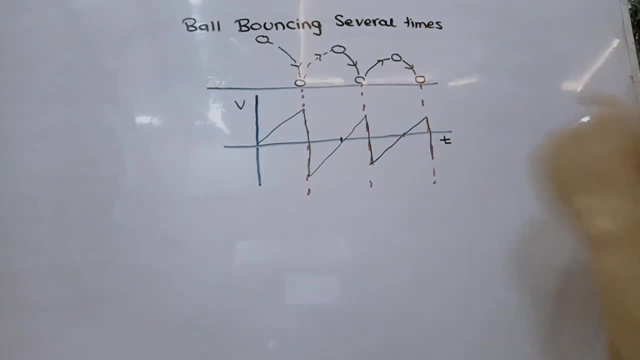 So let's start from this thing: The ball is moving, The ball is thrown from rest at. velocity is equal to zero. We have shown over here that velocity is equal to zero. over here It moves down towards the ground with constant acceleration. that is 9.81.. 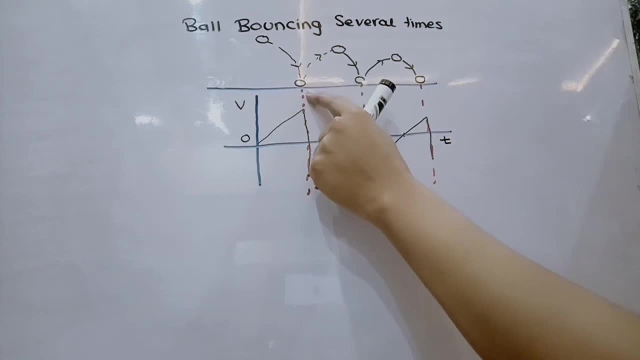 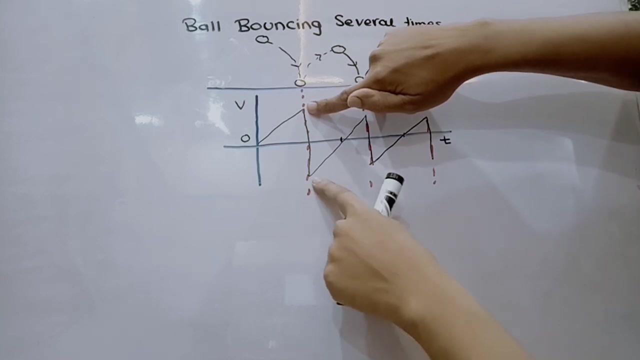 And when it impacts on the ground and changes its direction, the velocity, as it is a vector quantity, it changes its direction at the same time, although we can say that this, this change in direction, would take some milliseconds, but over here we are assuming that it takes zero seconds, although we can say that it can take a bit of a margin of time. 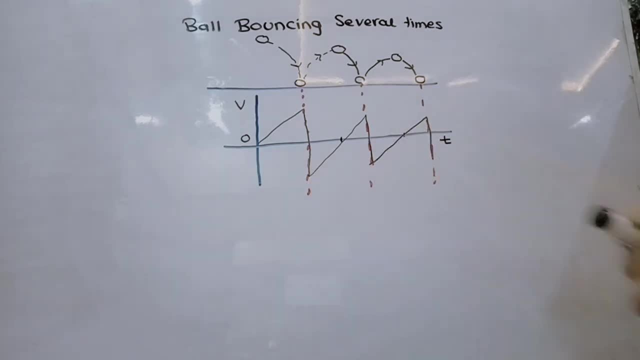 So over here, the direction changes. Now this is the place where the direction of the ball changes. So over here, the direction changes. Now this is the place where the direction of the ball changes. Here you can see that it increases and it turns upwards. 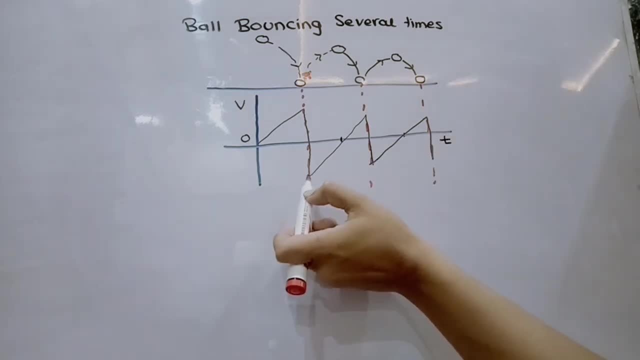 Now, this is the moment where it rises, And when it rises, it reaches its maximum height over here. That's the maximum height. At this maximum height, this velocity becomes zero because, as you all know, that at the maximum height the maximum potential energy is maximum. 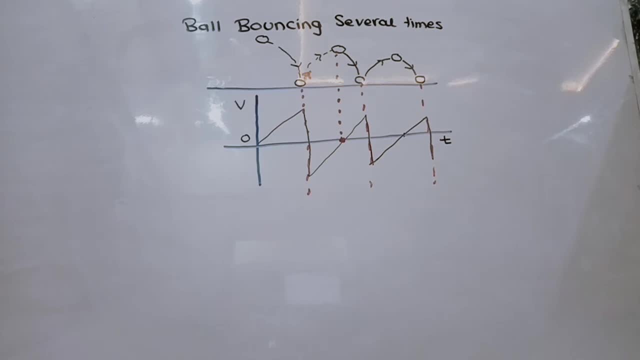 And the potential kinetic energy is zero. So that implies that this maximum height, at this maximum height, the performance will be zero. So we can simply label this: that in this interval it was rising, in this interval it was falling, and again in this interval it's again falling. It's over here. Now you must realize. 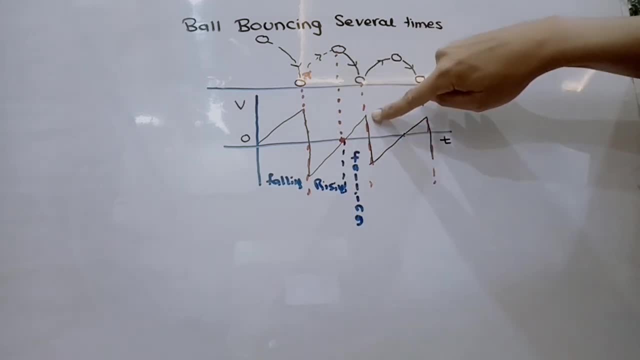 that after this, this peak velocity peak is less than this thing. So, as we know that the height decreases, So because of that the velocity decreases, As I have told you in the start, that kinetic energy also decreases, or the velocity also must decrease. So the same cycle again. 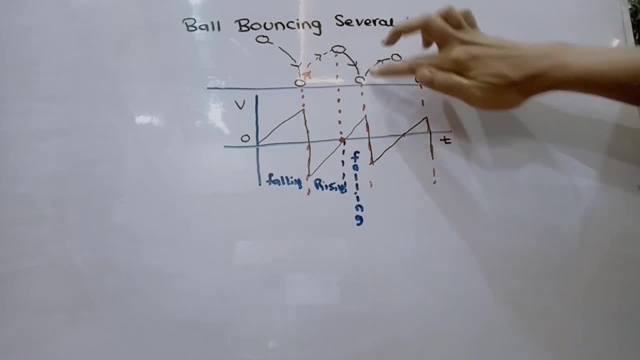 repeats It again, moves down, It again moves down. over here This shows that a downward movement, and over here the change of direction is shown by this line. So again it moves upward with the lower velocity, and then again it continues, and so on. So after this, what we can do is discuss. 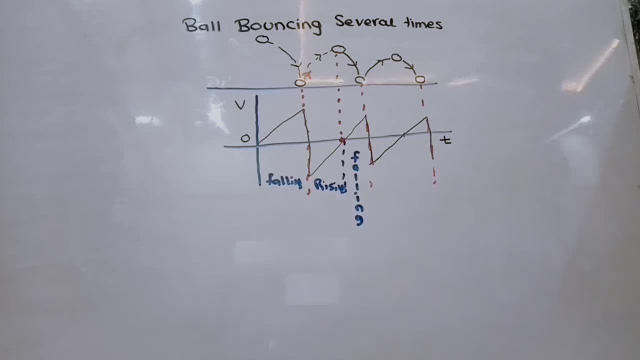 the acceleration time graph For this case. now for the acceleration time graph. you can clearly see the acceleration is constant, but what we have to do is that, for example, in this interval it's falling, It's with a constant acceleration. This is the constant acceleration, but during this impact there would